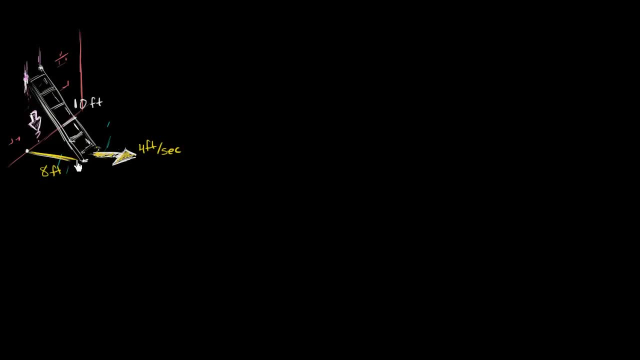 So if we call the distance between the base of the wall and the base of the ladder, let's call that x. We know right now x is equal to eight feet. We also know the rate at which x is changing with respect to time. 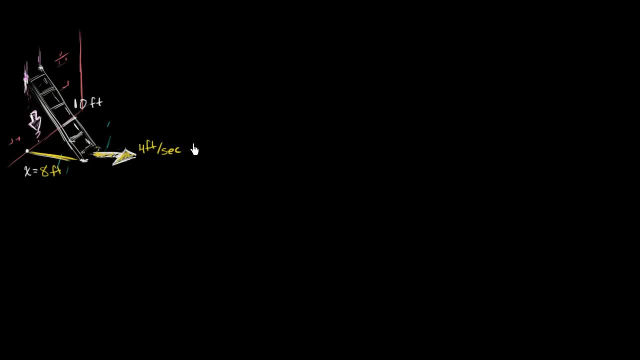 The rate at which x is changing with respect to time is four feet per second, So we could call this dx- dt. Now let's call the distance between the top of the ladder and the base of the ladder h. Let's call that h. 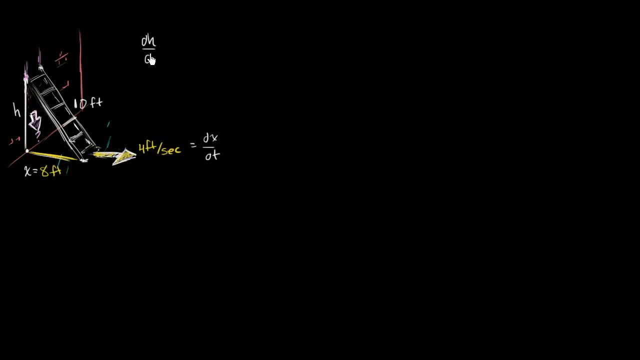 So what we're really trying to figure out is what dh, dt is, given that we know all of this other information. So let's see if we can come up with a relationship between x and h And then take the derivative with respect to time. 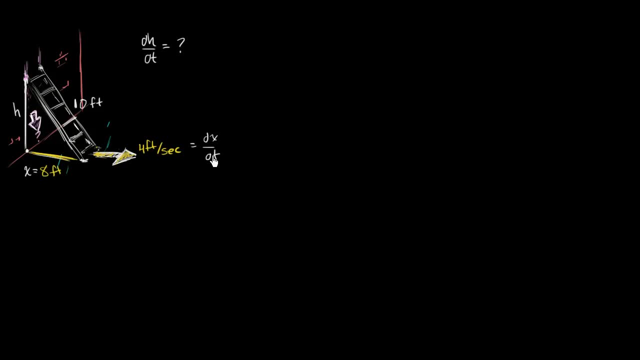 maybe using the chain rule and see if we can solve for dh, dt, dh, dt. knowing all of this information Well, we know the relationship between x and h at any time because of the Pythagorean theorem, We can assume this is a right angle. 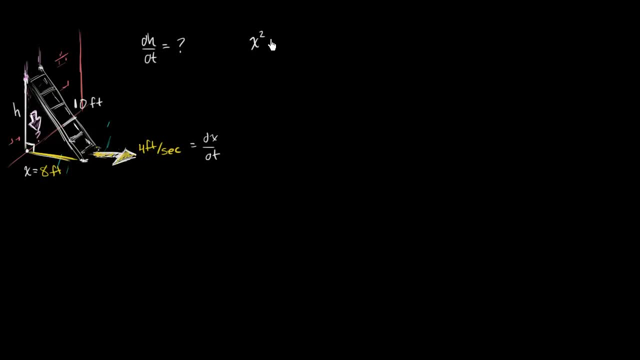 So we know that x squared plus h squared is going to be equal to the length of the ladder squared, It's going to be equal to 100.. And what we care about is the rate at which these things change with respect to time. So let's take the derivative with respect to time of both. 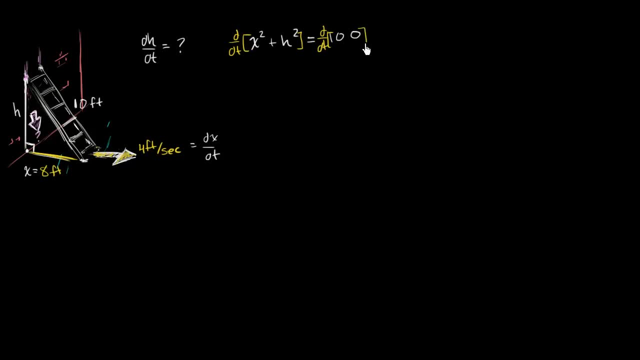 sides of this. So we're doing a little bit of implicit differentiation. So what's the derivative with respect to time of x squared? Well, the derivative of x squared with respect to x is 2x, And we're going to have to multiply. 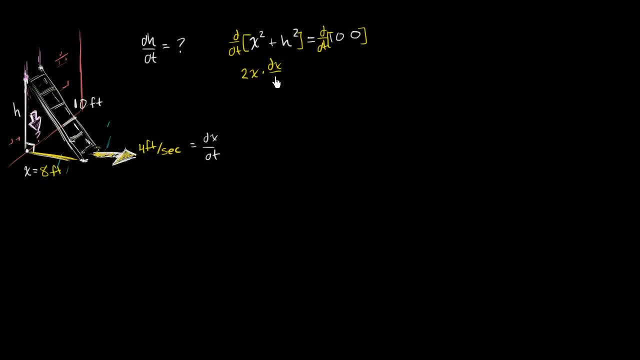 that times the derivative of x with respect to t, dx, dt. Just to be clear, this is a chain rule. This is the derivative of x squared with respect to x, which is 2x times dx dt. to get the derivative of x squared with respect to time, just the chain rule. 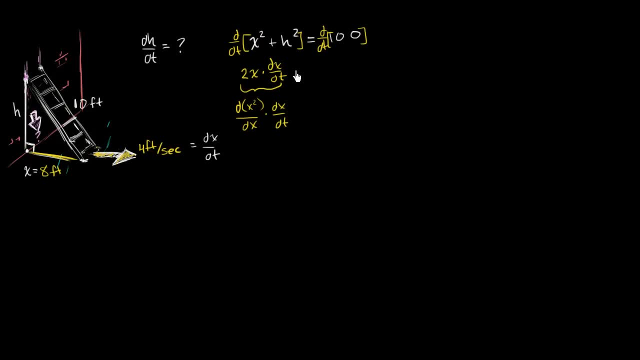 Now, similarly, what's the derivative of h squared with respect to time? Well, that's just going to be 2h. The derivative of h squared with respect to h is 2h times the derivative of h with respect to time. Once again, this right over here is the derivative. 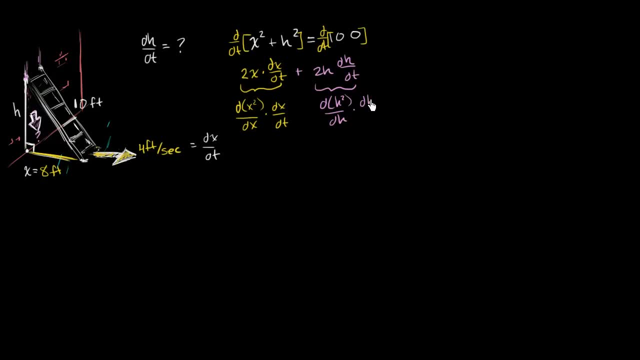 of h squared with respect to h times the derivative of h with respect to time, which gives us the derivative of h squared with respect to time. And what do we get on the right hand side? What do we get on the left hand side of our equation? 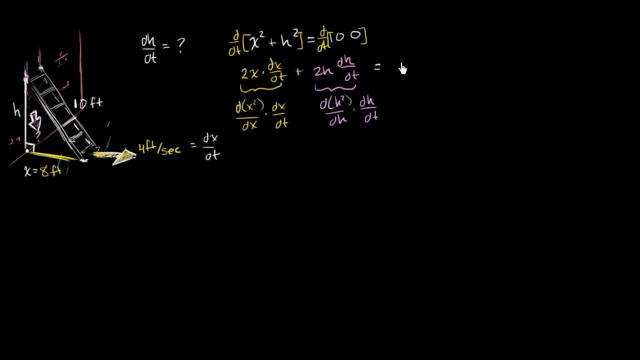 Well, the length of our ladder isn't changing. This 100 isn't going to change with respect to time. The derivative of a constant is just equal 0. So now we have it: a relationship between the rate of change of h with respect to time. 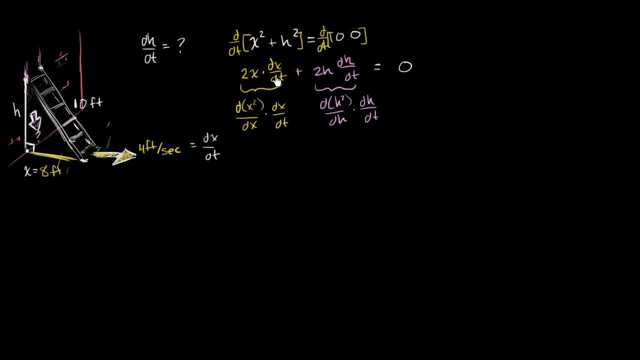 the rate of change of x with respect to time and then at a given point in time, when the length of x is x and h is h. But do we know what h is when x is equal to 8 feet? Well, we can figure it out. 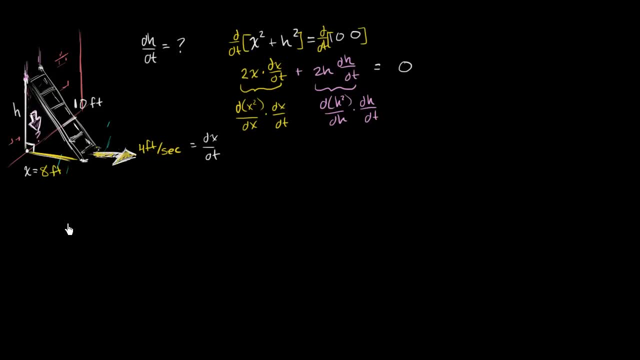 When x is equal to 8 feet, we can use the Pythagorean theorem. Again, we get 8 feet squared plus 8 squared is going to be equal to 100.. So 8 squared is 64.. Subtract it from both sides. 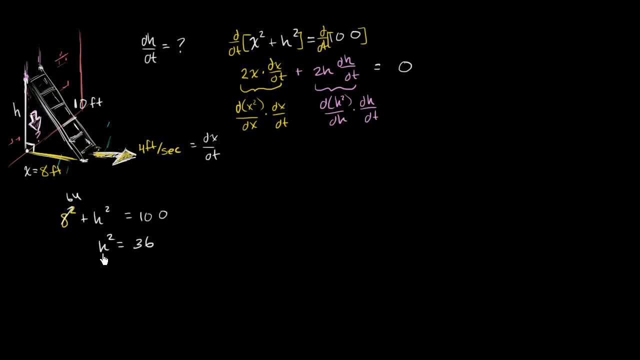 You get 8 squared is equal to 36.. Take the positive square root. A negative square root doesn't make sense because then the ladder would be below the ground. It would be somehow underground. So we get h is equal to 6.. 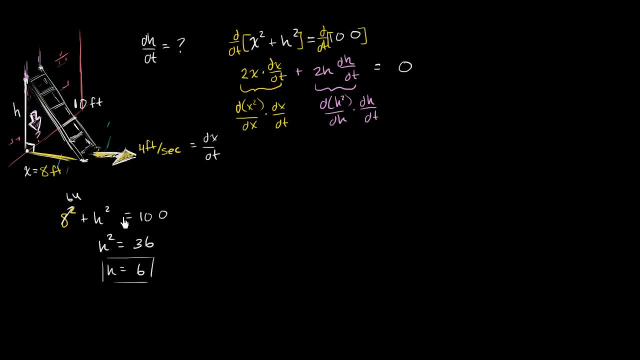 So this is something that was essentially given by the problem. So now we know, We can look at this original thing right over here. We know what x is. That was given. Right now x is 8 feet. We know the rate of change of x with respect to time. 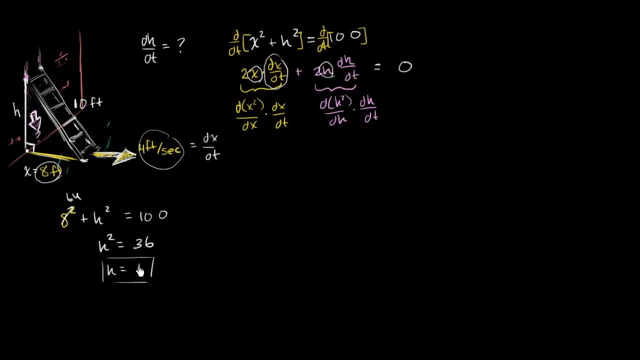 It's 4 feet per second. We know what h is right now: It is 6.. So then we can solve for the rate of h with respect to time. So let's do that. So we get 2 times 8 feet, times 4 feet per second. 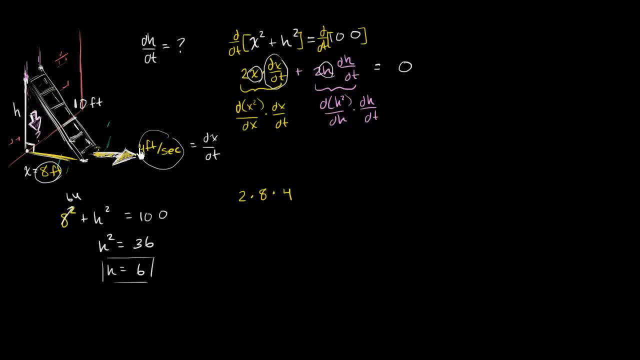 So times 4 plus 2h, So plus 2h is going to be plus 2 times our height. right now is 6, times. the rate at which our height is changing with respect to t is equal to 0. And so we get 2 times 8. times 4 is 64 plus 12 dh dt. 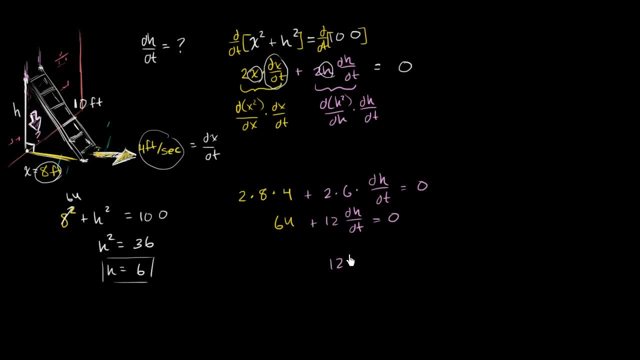 is equal to 0.. We can subtract 64 from both sides. We get 12.. 12 times the derivative of h with respect to time is equal to negative 64. And then we just have to divide both sides by 12.. 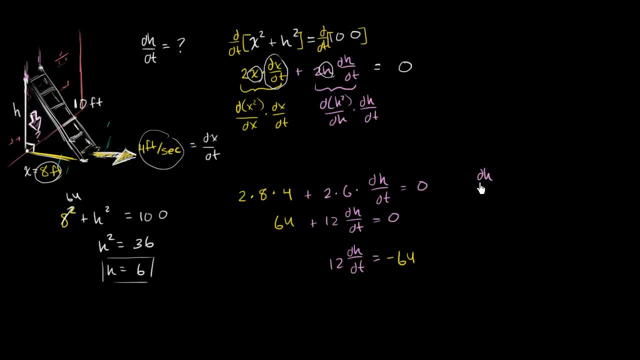 And so now we get a little bit of a drum roll. The derivative, the rate of change of h with respect to time, is equal to negative 64. divided by 12, is equal to negative 64 over 12,, which is the same thing as negative 16 over 3..